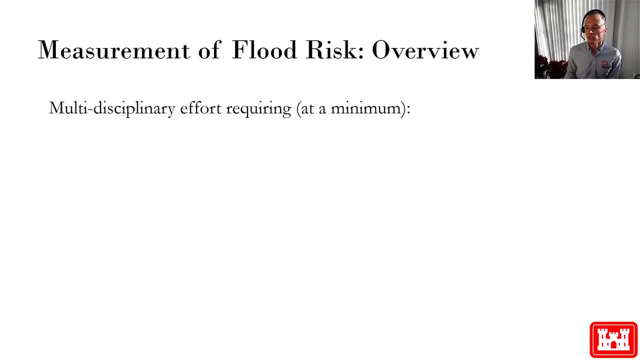 The planner should also be heavily involved In a holistic view. planners should be competent enough of an engineer and economist with sufficient enough understanding of the models, such as RAS, FDA, HMS, such that the planners can help engineers and economists select compatible and cost-effective methods and models. 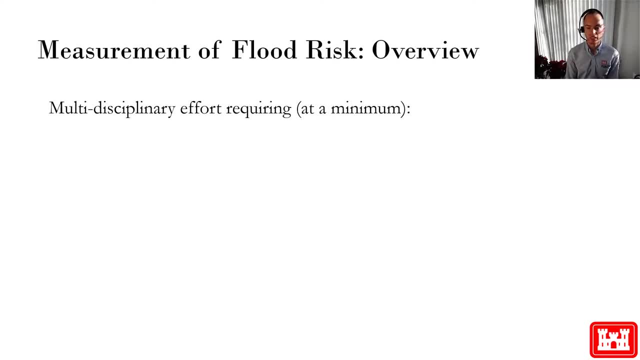 for example, collecting a sample or completing a survey using steady or unsteady hydraulics, using the Rational Method or SCS curves, The planner will define with the local sponsor and the project delivery team the water resource problem being solved. 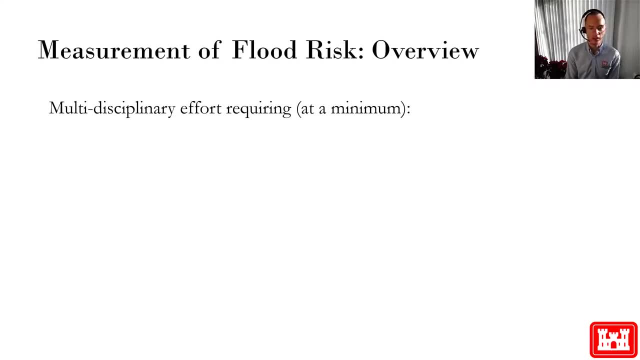 Is it a flood problem? Do we, the Army Corps of Engineers, have the legal authority to address the problem as a federal agency, or is it statutorily a local, state or other federal agencies' responsibility? Is it a flood problem? 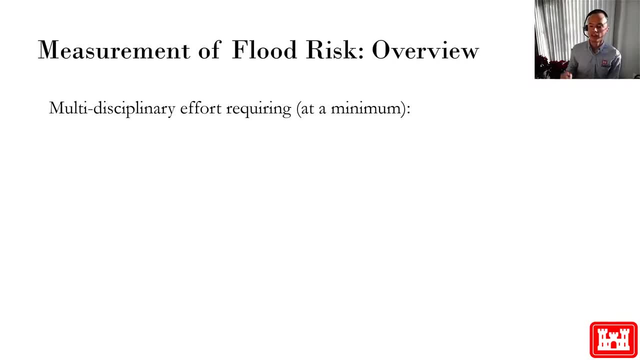 Do we, the Army Corps of Engineers, have the legal authority to address the problem as a federal agency, or is it statutorily a local, state or other federal agencies' responsibility? The planner will also lead the team toward developing a scope of work schedule, study objectives and the study area boundaries. 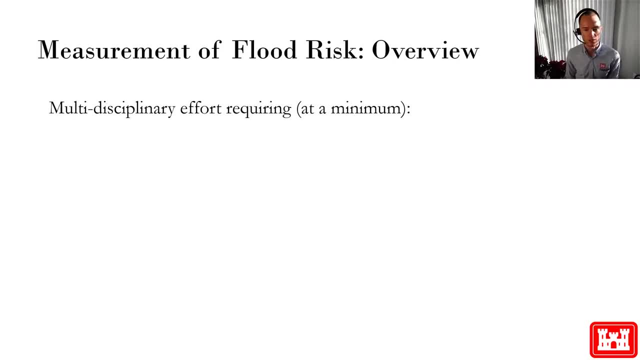 Later in the process, the planner will lead the team through the development of potential water resource solutions which are the alternatives. Hydrologists study the spatial and temporal distribution of water. Hydrologists study the spatial and temporal distribution of water. Hydrologists cannot say specifically that a world-wide Mariupol study is a work-life balance. 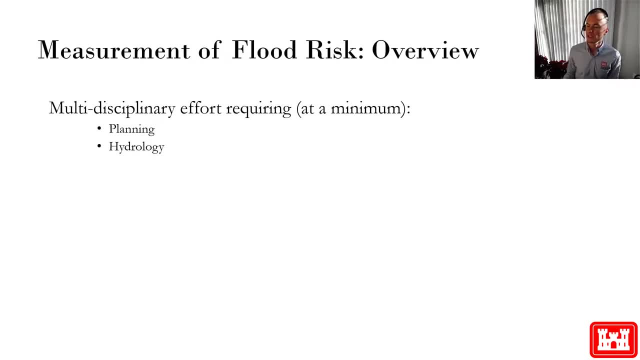 Hydrologists cannot say specifically that a world-wide Mariupol study is a work-life balance, if it will rain, let alone flood, tomorrow or next year, but hydrologists can provide you with a probability that it floods. The output you're usually looking for is a probabilistic description of the annual 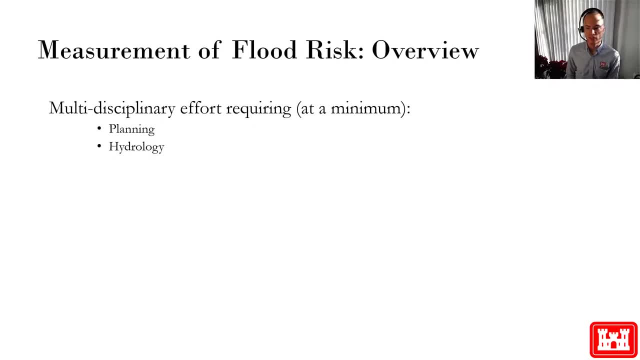 peak flow of water in a stream at various locations within the study area for expected annual damages computations For dam and levee safety studies. you are looking for the stream flow for a given event. You may be interested in an entire storm's hydrograph if you're concerned with life. 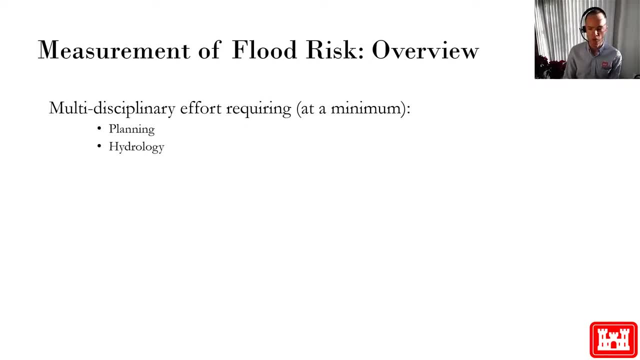 loss, regional economic losses, agricultural damages or traffic delays. Hydraulic engineers study the physical properties of water and, in our case, the movement of water through open-air channels and the floodplain. The output you're often looking for from hydraulic engineers is the stage, the topographic. 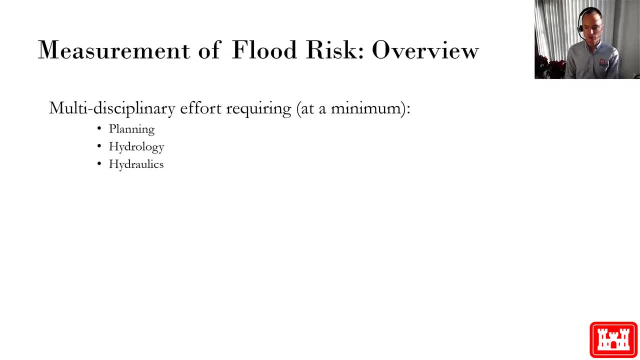 elevation of water. You may be interested in water for a given or range of flows provided by the hydrologist. Sometimes you might also be interested in velocities and an entire hydrograph for dam and levee safety. The economist provides decision support information. 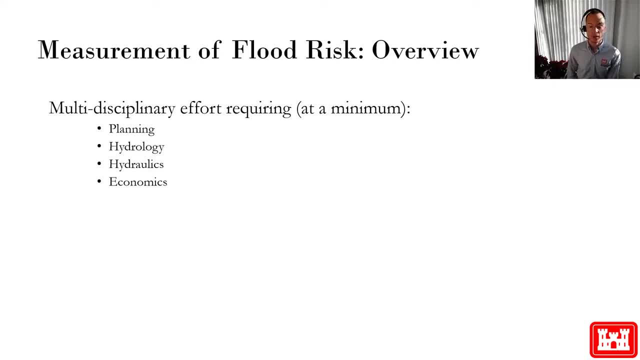 You'll be studying the consequence, damage or life loss associated with a given hydraulic condition- the stage. You'll also be supporting the evaluation and selection of a plan, but we'll get there later. You are likely to depend on others to complete your analysis. 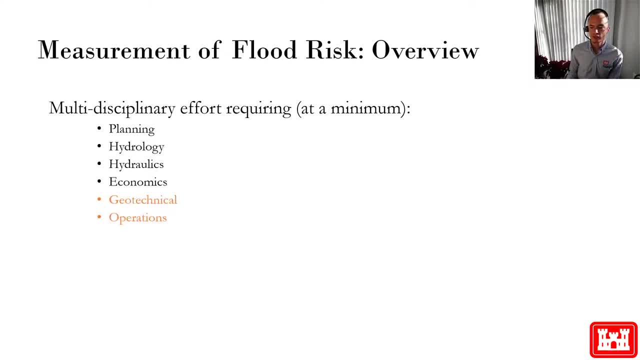 In terms of risk assessment: geotechnical engineers describe the probability of levee or bank failure for a given stage and water managers describe the operations at existing structures for a given or range of storms. In the last video of this series, we will discuss how cost engineering and real estate 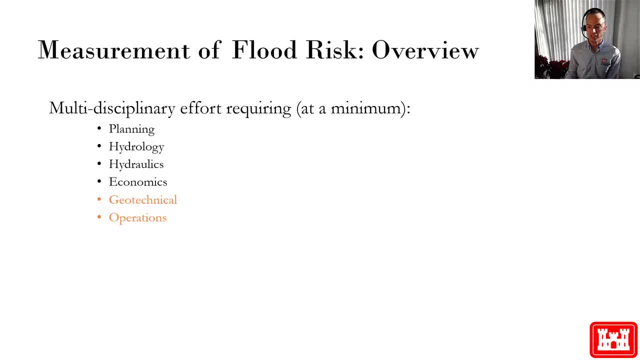 come into play. but first let's discuss expected annual damage, or EAD, as a measurement of risk. Expected annual damage measures damages to structures and infrastructure as a result of flooding, which forms the basis for most planning-level decisions. Now we have looked at briefly how each of these disciplines come into play. In the last video of this series, we will discuss how cost engineering and real estate come into play. but first let's discuss expected annual damage, or EAD, as a measurement of risk. In the last video of this series, we will discuss how cost engineering and real estate. 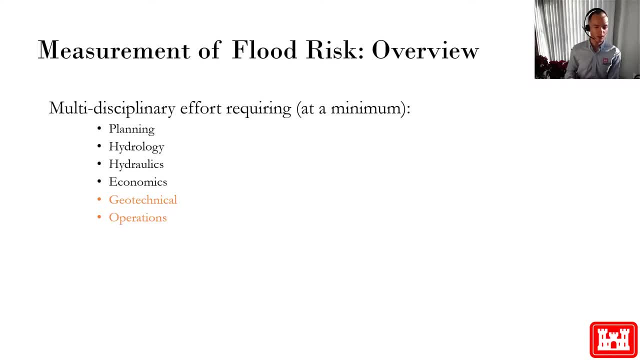 come into play. but first let's discuss expected annual damage, or EAD, as a measurement of risk. In the last video of this series, we will discuss how cost engineering and real estate come into play. In the next video of this series, we will discuss how cost engineering and real estate Let's 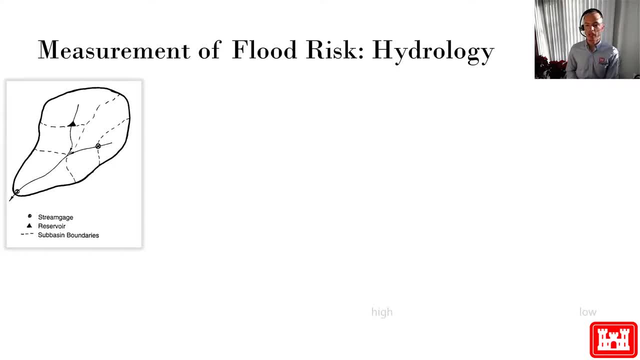 look into each of these disciplines in a little bit more detail. Hydrologists may create a rainfall runoff model or perform a frequency analysis of flow records For FIA. hydrologists will provide a hydrograph the flow as a function of time relationship. 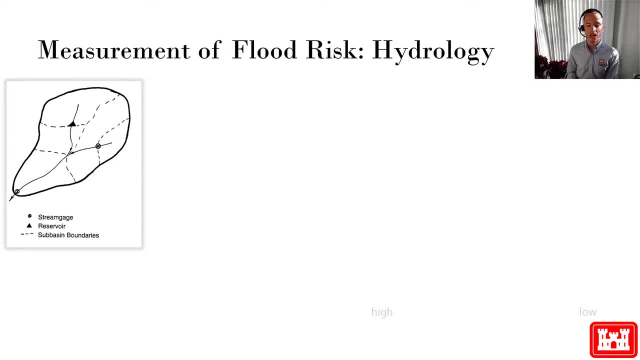 For FDA, we model damages as a function of annual peak flow or state. For example, FIA uses the cathode as a function of the annual peak flow or state. So just the top of the tallest hydrograph, tallest hydrographic frequency, as illustrated using the dashed lines in the middle image. 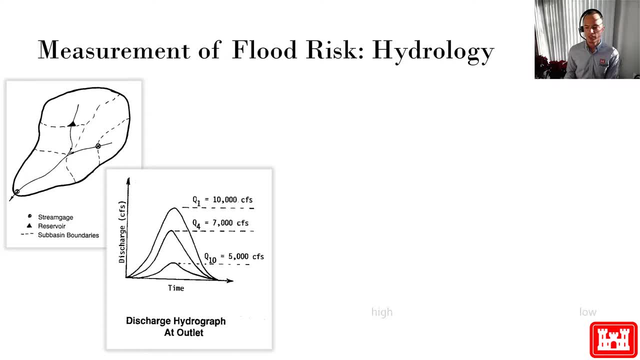 In other words, we are concerned with the relationship, as in the diagram on the right that tells us the probability, measured on the x-axis, that a given flow measured on the y-axis is exceeded in any given year. This diagram is simply a cumulative distribution function, except that the x- and y-axis are 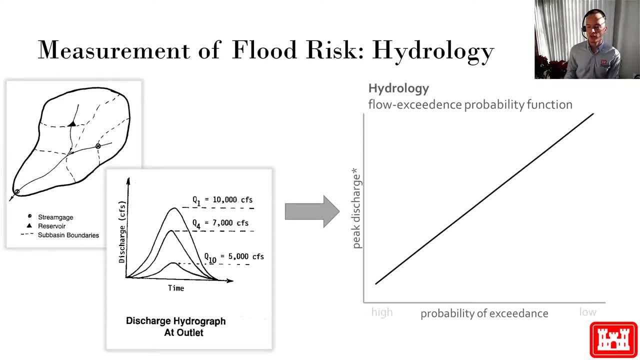 flipped. A typical CDF would show probability on the y-axis as a function of flow, but we are looking at the probability that a flow is exceeded, In other words, the flow being greater than 0.. A typical diagram will show the opposite: the probability of non-exceedance. 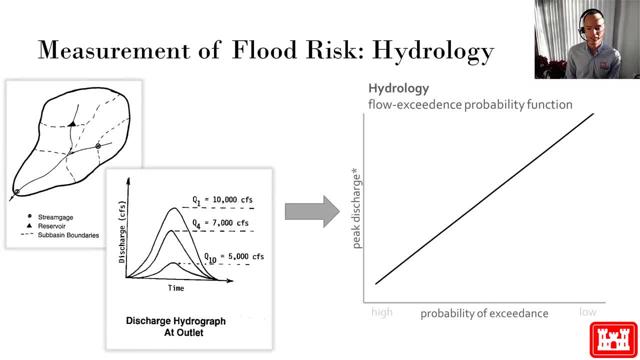 The other unique thing about this diagram is that the x-axis is in reverse order, so that the graph is upward sloping with lower probabilities on the far end of the axis. So a flow with a 50% chance of exceedance in any given year, or about a 2-year storm, has a low flow rate. So a flow with a 50% chance of exceedance in any given year, or about a 2-year storm, has a low flow rate. A flow with an upward slope of 100% as a reflection of flow is chilling and marbling. 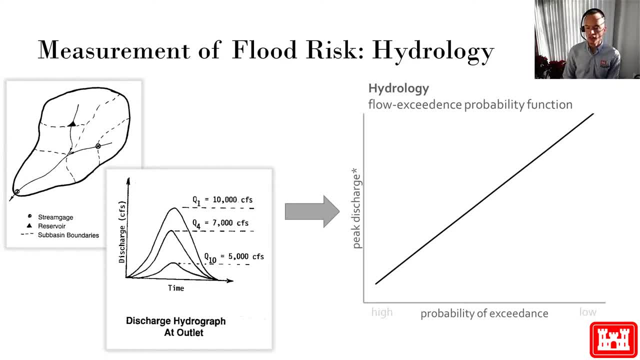 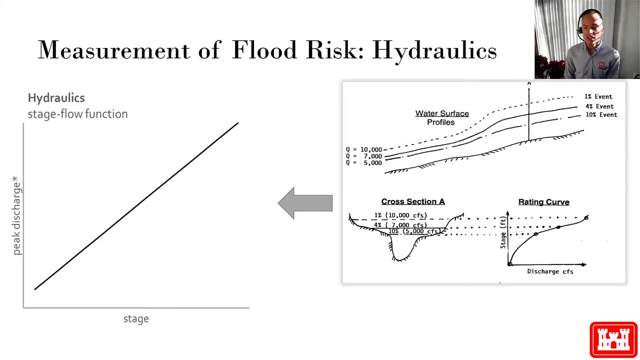 at top speed per second, Not in this diagram, would we have done a high flow rate. The only unknown right answer is a high flow, which might be a confrontational flow factor, but by referring to the diagram giving the last option is the revolution. 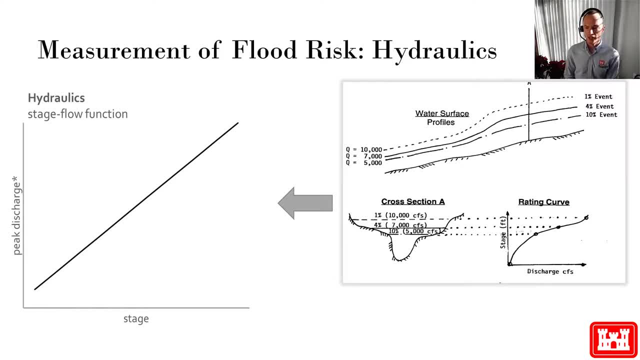 And I'm not really going to go so far as to tell whether or not this diagram is consistent or not, But it's a good suggestion to actually think about before you had to go for and use嗎, and later use it with examples such as waves at low tide treatment. 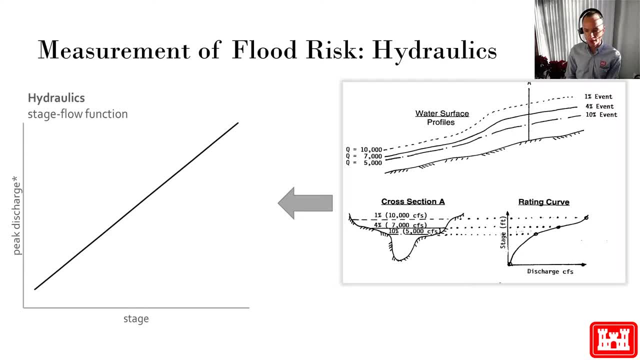 And this is why imagine that you have to compare the graph in reverse. Where does water go in the floodplain? And this also has to do with things like channel roughness that affect the velocity of the flow. How quickly can the water be routed? 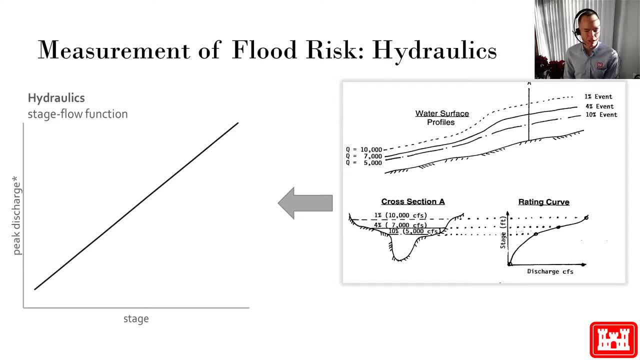 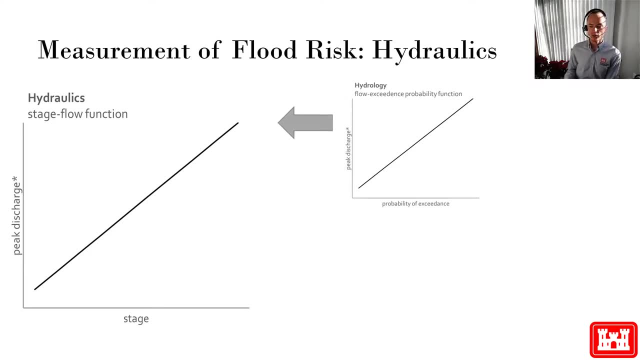 Does the water rush by or does the water get stuck and back up? And now you get to see why we invert the flow frequency axes For a given frequency event, such as a storm so large that 99% of events produce smaller flows. 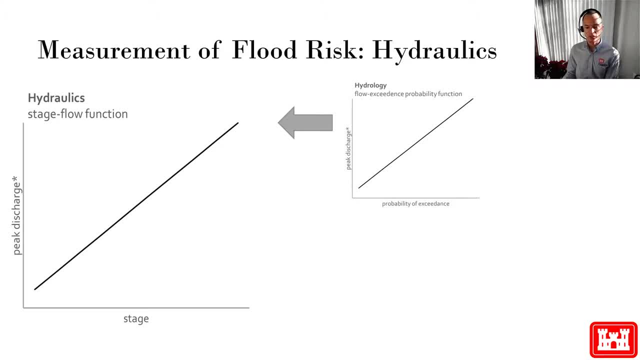 the 1% annual chance of exceedance event, we can calculate flow And for a given flow, we can calculate the river stage, the water surface elevation or depth of flooding. We ask economists to tell us, for a given stage or water surface elevation, how much damage would be produced. 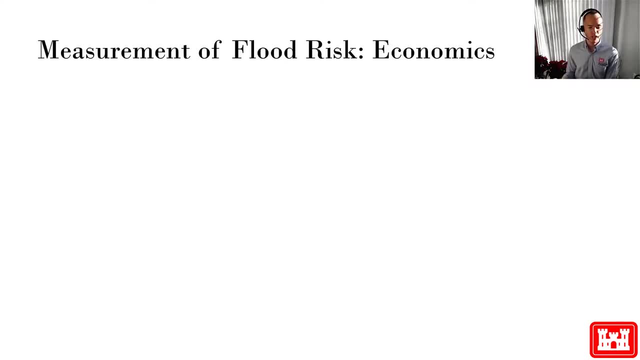 This involves tying together information from different sources. We start with terrain. We start with terrain or topographic data, and this gives us ground elevations. The ground elevations are linked to structure locations and this gives us the ground elevation at each structure. 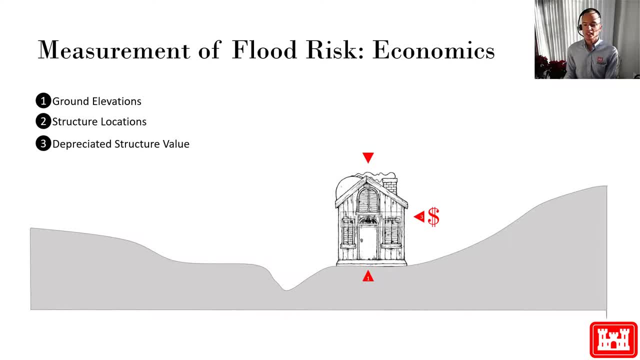 The structures have values and we care about the structure's value and its current condition, which is the depreciated structure replacement value. Structures also have other attributes, such as structure use. We collect information which helps us to generalize some information about the value of the structure's contents. 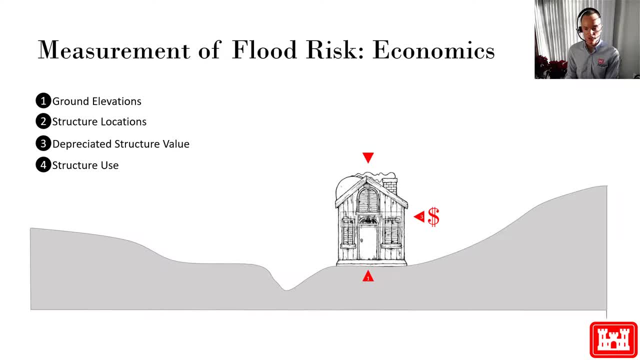 the structure's likely method of construction and therefore susceptibility to damage. We also generalize some uncertainties and other point estimates, such as the number of vehicles at each structure using the structure's use. Finally, we collect information about the elevation of structures. 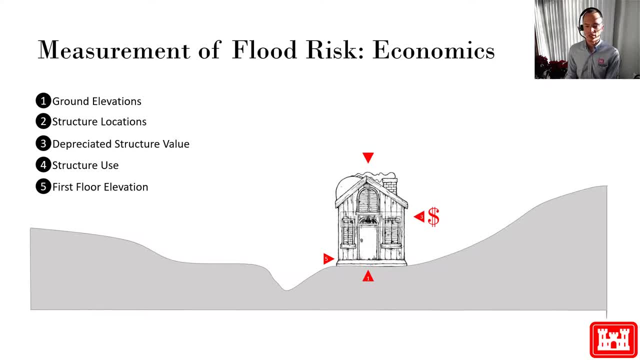 which gives us the elevation of the structure's volume and the value of the structure's growth over time at which water enters the structure. This information is linked to hydraulic data, which describes the depth of floodwaters in the floodplain. This accomplishes our main goal. 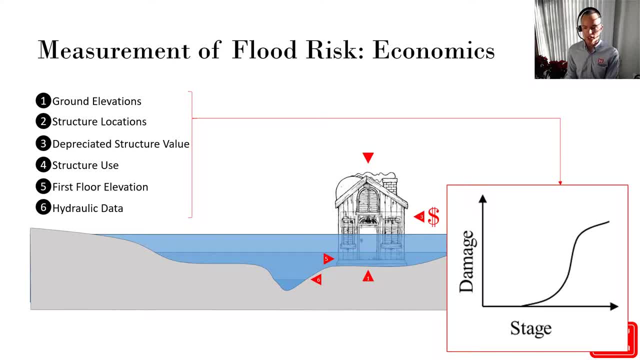 which is the development of a percent value damaged stage relationship. This relationship can be applied to a wide range of events. The percent damage information generally comes from expert elicitation, direct observation or a mixture of both. The depth damage information is aggregated by impact area or reach. 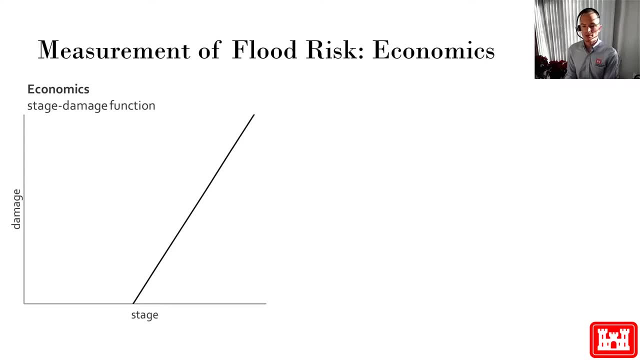 For a given location where water breaks out and begins to flood infrastructure. we now know that for a given frequency event, how large the flow will be, For a given flow, how high the water will be And, for a given stage, how much damage there will be. 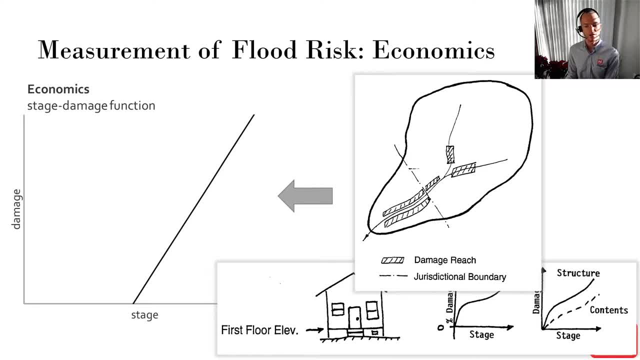 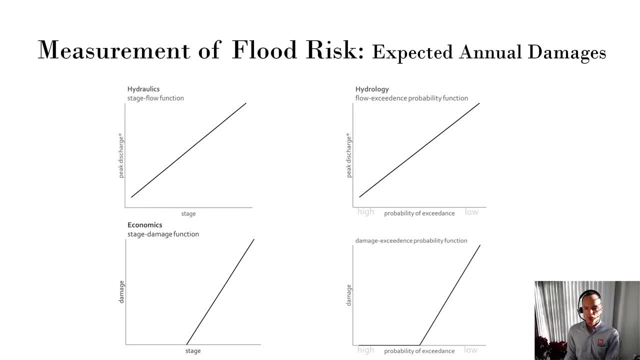 You can now start to see how this Monte Carlo process allows us to analyze how uncertainties in the input parameters affect our output parameters, the damages. So let's follow this process through: Starting with a given frequency event, we calculate the flow. From this flow, we calculate. 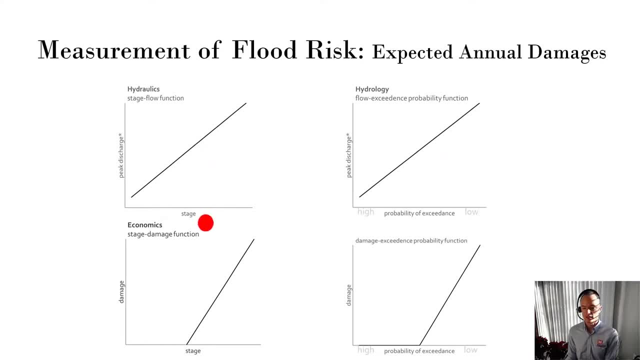 the stage. From this stage we calculate the damage And thus we can calculate the probability of a given value of damage. Let's back that up real quick. We calculate the flow from the flow exceedance probability function And from that flow. 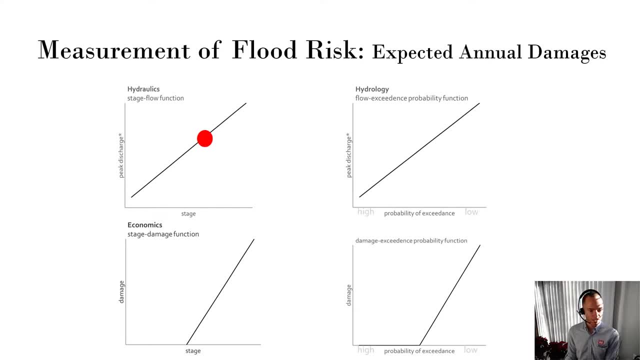 we calculate the stage from the stage flow function, also known as the rating function. From that stage, we calculate a damage from the stage damage function, And that information gives us, together with the flow exceedance probability function, a damage exceedance probability function. 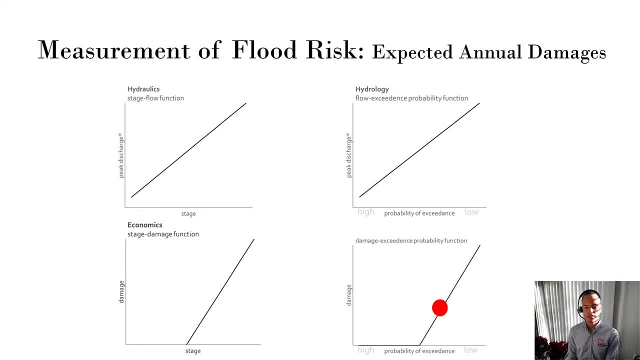 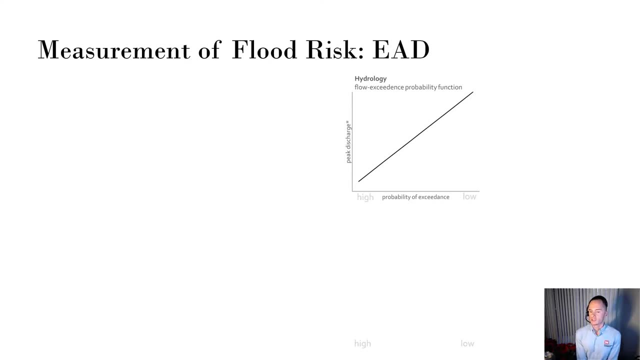 This methodology importantly assumes that we can measure damage as a function of stage. The way that I just described FDA's calculation is the most intuitive way to understand the program and is sufficient for non-economists. However, we do not randomly sample events in FDA. 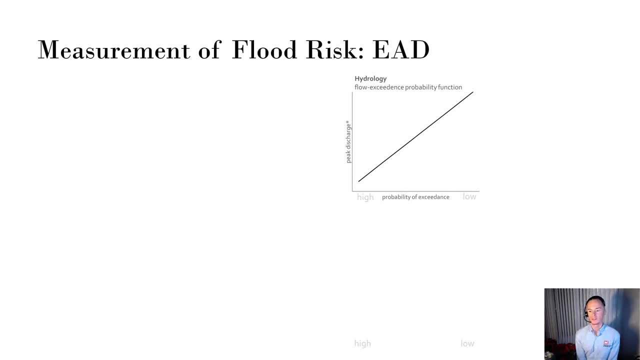 We randomly sample curves. There is uncertainty about each of these relationships, So rather than look at an event at a time, we look at a curve at a time, And this makes our expected annual damage calculation seem more straightforward. Let's take a look at this. 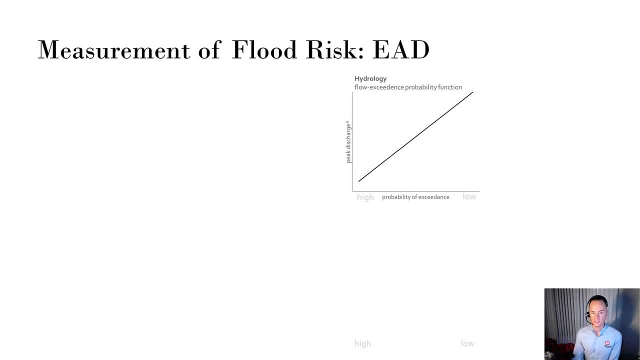 First, we randomly select a flow exceedance probability function, We randomly select a stage flow function, a stage damage function, and these three functions together produce a realization or an instance of a damage exceedance probability function and the integration of which produces a realization of expected annual damage. 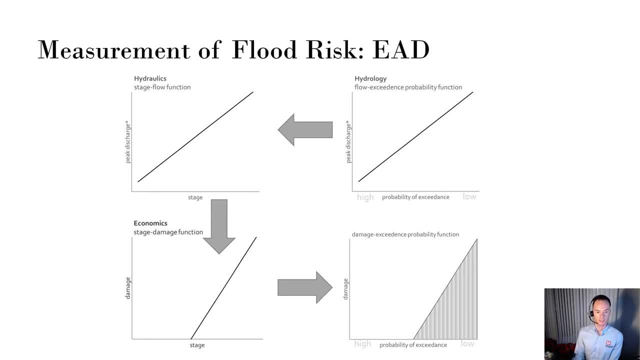 Each time that we randomly select a different set of functions, we get a different damage exceedance probability function and a different realization of expected annual damage. What are some things that we can say about expected annual damage? Our measurement of flood risk in general? 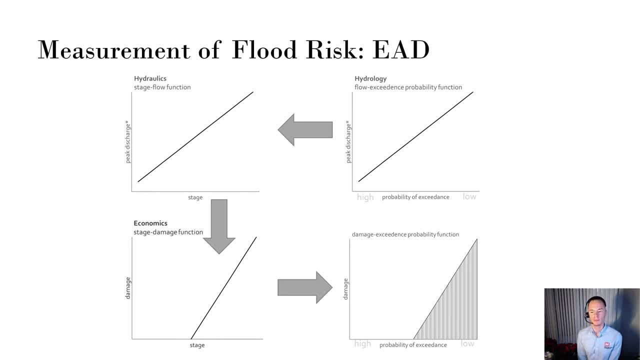 Well, expected annual damage is a probability-weighted average amount of flood damages that one would expect to experience in any given year, without a priori knowledge about whether or not any flooding will occur in that year. Since flood events are, by their very nature, rare events, expected annual damage will generally overestimate the damages. 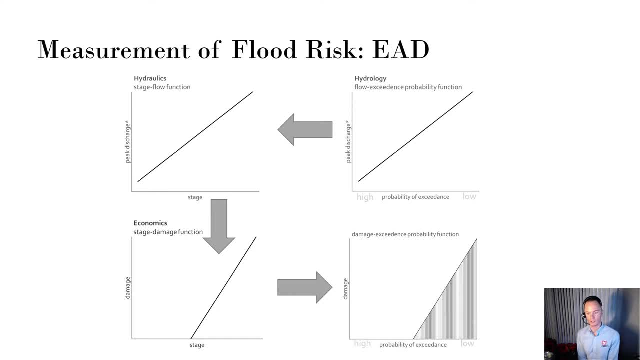 occurred in that year. Since flood events are, by their very nature, rare events, expected annual damage will generally overestimate the damages occurred in that year In most years- since there will be no damage in most years- while simultaneously underestimating the damages that will be incurred after most flood events. 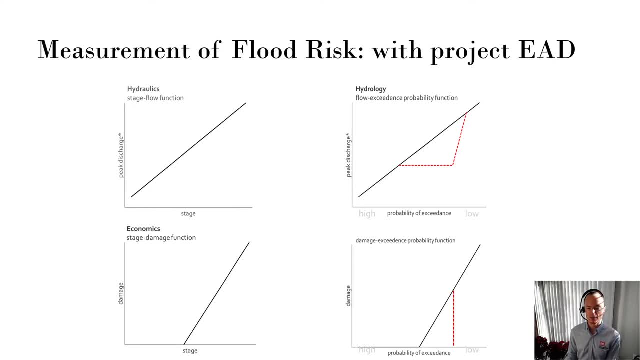 Let's consider an alternative that proposes building a dam. The dam would hold back flow near some town, such that for large events or low-frequency events, peak flows are reduced. This continues until the dam would become dangerously full, at which point releases would increase For a given flow. the stage would stay. 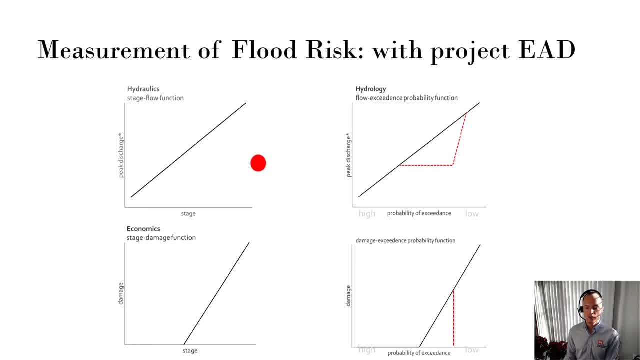 the same. In other words, the river channel, in this case, has not been changed. For a given stage, damages are the same, assuming the dam does not encourage or discourage development. But because we have decreased the frequency of certain peak stages, we have truncated the damage frequency.